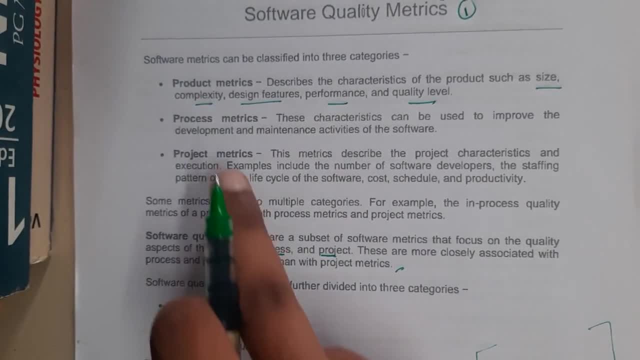 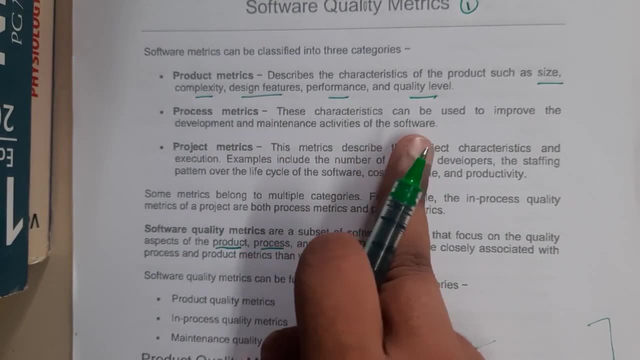 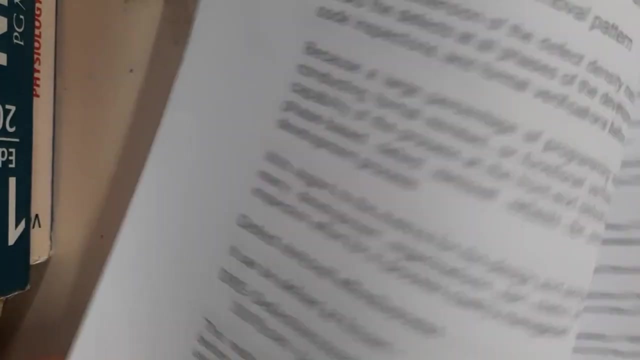 are some properties you can say which are showed in product matrix, Similarly what are shown in process matrix. So these characteristics can be used to improve the development and maintenance activity of the software. So basically, in process matrix defects will be shown, guys. Okay, so we'll be discussing about those defects And 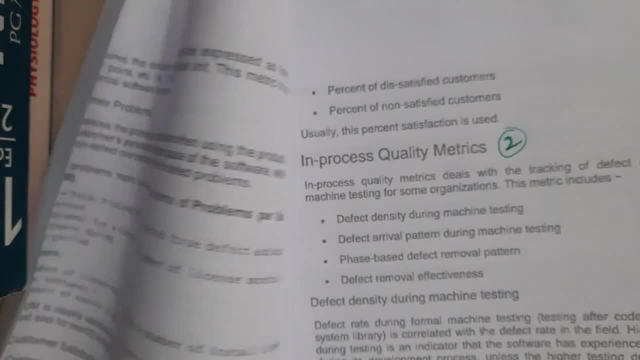 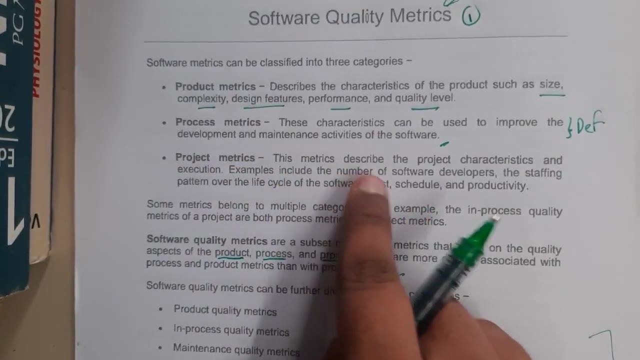 so I think there are three types of, four types of defects. we will be discussing them in our next lecture, guys don't worry. Okay, yes, Similarly in project matrix. So this matrix that describes the project, characteristics and execution. Okay, so what is the cost of execution? What is the time? 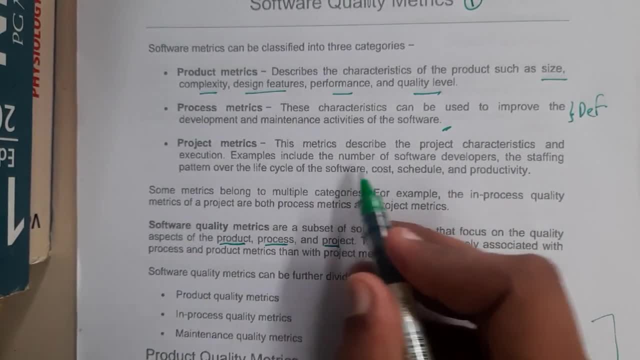 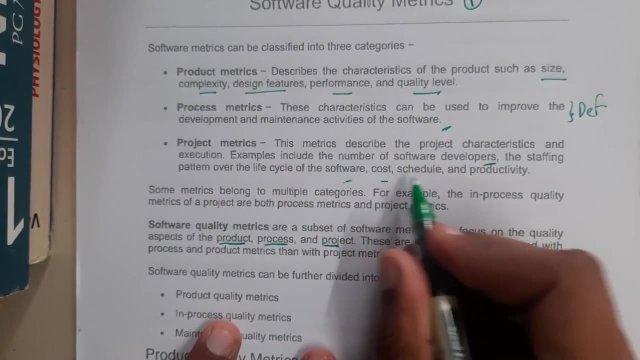 time lifecycle, So how many developers are needed, So all these things. So example, it includes the number of developers was used- The staff pattern over the life cycle, like how many hours they are working in that way, similarly cost schedule and productivity. so these all things will. 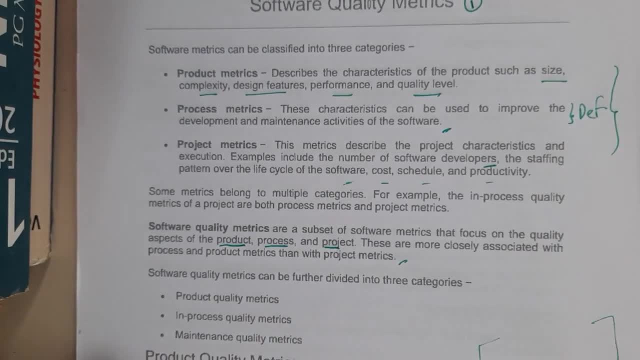 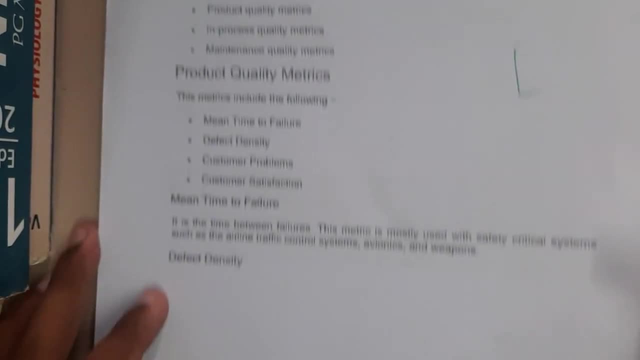 be shown, guys. so now i hope everyone got some basic idea about the three different types of matrices, right? yes, so in this lecture let us continue with the product matrix, guys. okay, yes, so product matrix. so it basically includes these four characteristics. in simple words, you can say: 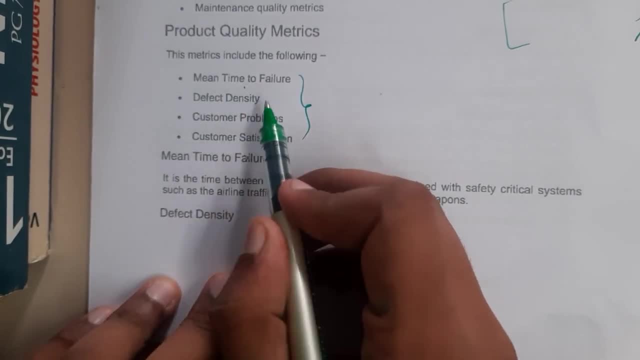 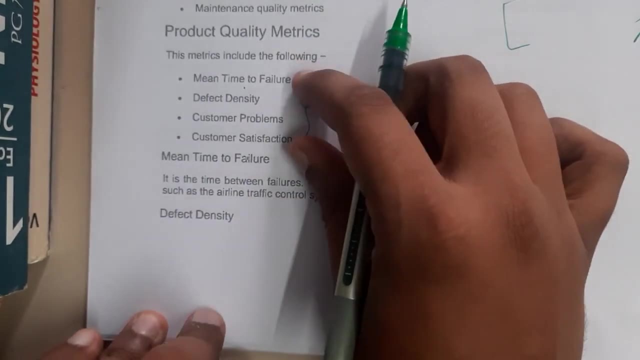 okay, so the first characteristic is nothing but mean time to failure. the second is a defect: density. the third is a customer problem. the fourth is customer satisfaction guys. these terms are literally self-explanatory. guys. you can understand just by the terms itself. okay, yes, so basically. 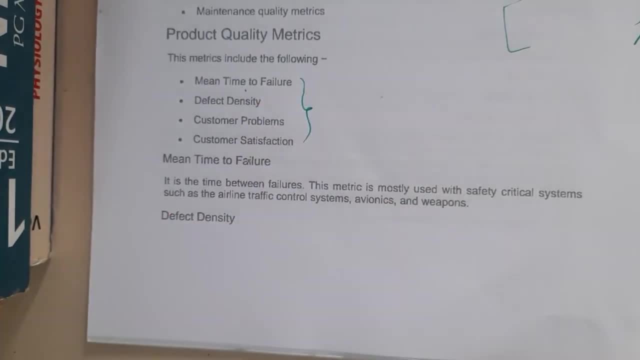 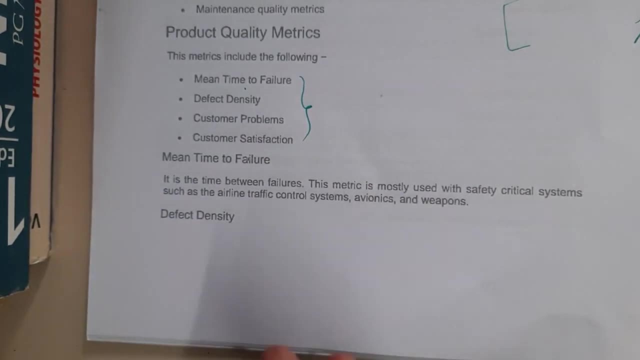 mean time to failure. so basically, what is the mean, guys? so mean is nothing but in between two, right, yes, so that is nothing. but if you are doing for the time of failure, so that concept is nothing but the mean time of failure, so it is the time between failures. the matrix okay is mostly used. 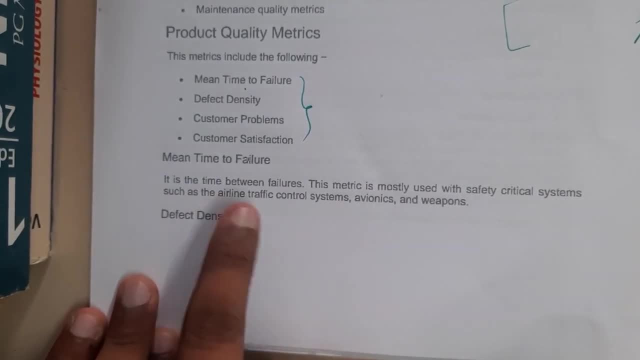 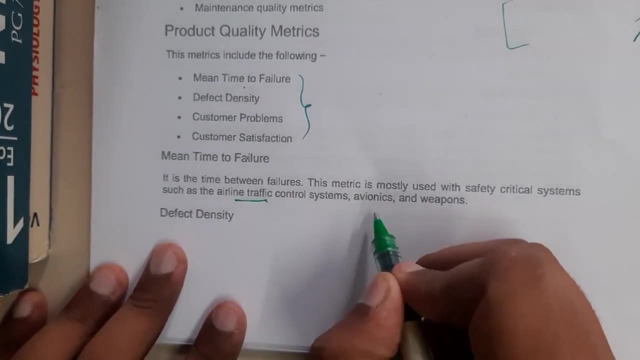 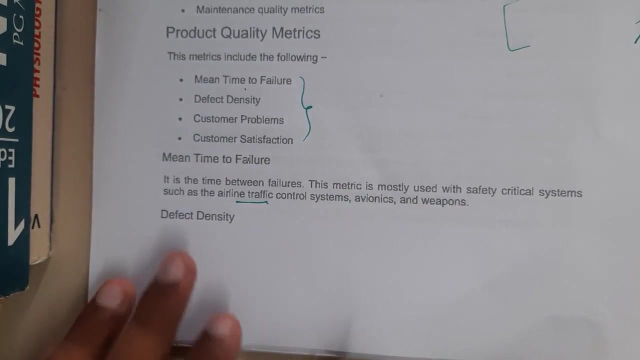 with the safety criteria system, such as airline traffic control or system. so basically, where time is really important, okay. so, like airlines or any kind of weapons, in those the time is really important, right. so at that places they will be using this matrix, okay, yes, similarly, defect density: okay. so let me go through. 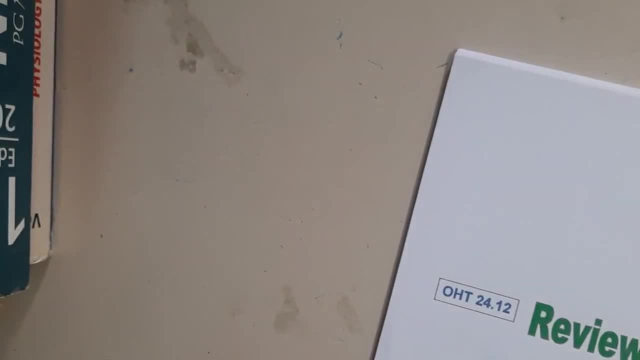 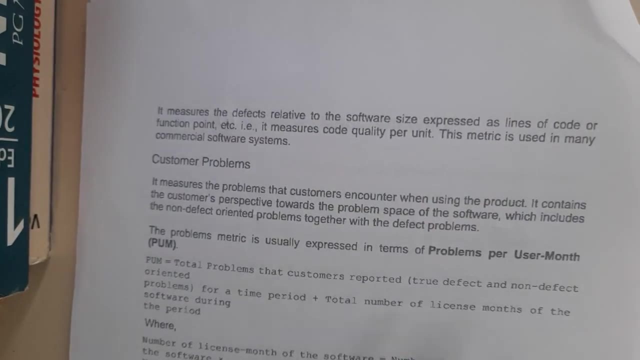 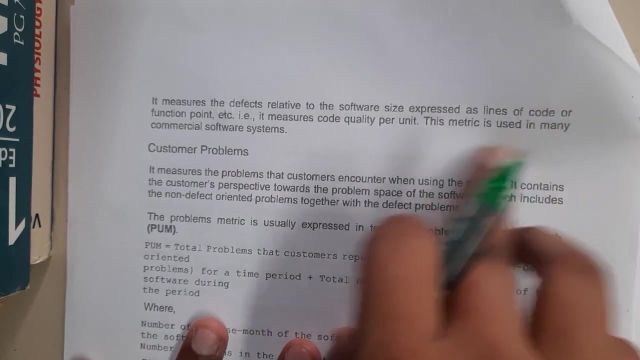 the theory. just give me a second, guys. i think all these answers have been collected from tutorial point- i'm not sure, but mostly it's from tutorial point- or greeks for greeks. guys, i think it's tutorial points only. okay, yes, so it's. it measures the defect related to the software size expected as a lines of code, or 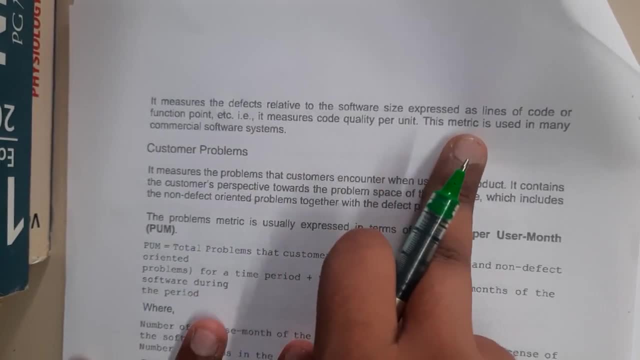 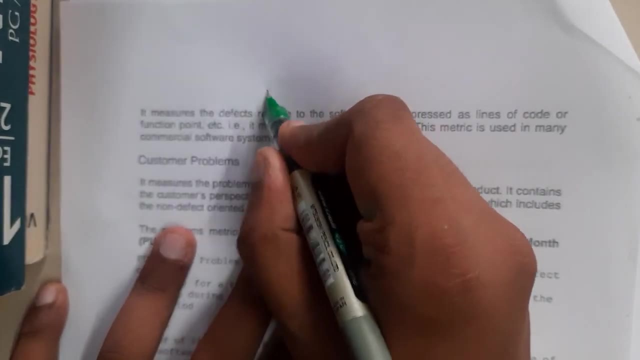 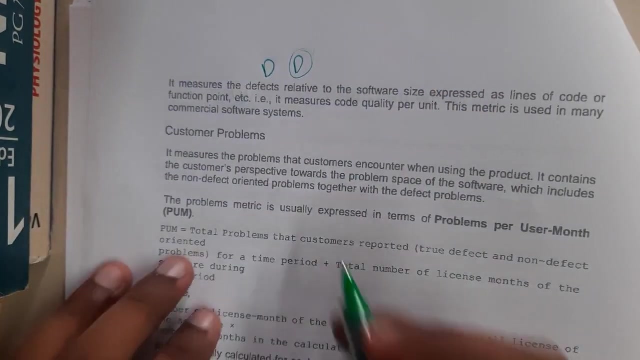 function points it measures the code quality per unit. okay, so this matrix is used in many commercial software systems. so if you recall the name, it is nothing but a density guy, right? so it is defect density. so basically, in some lines of code, what is the density of defects? so that thing. 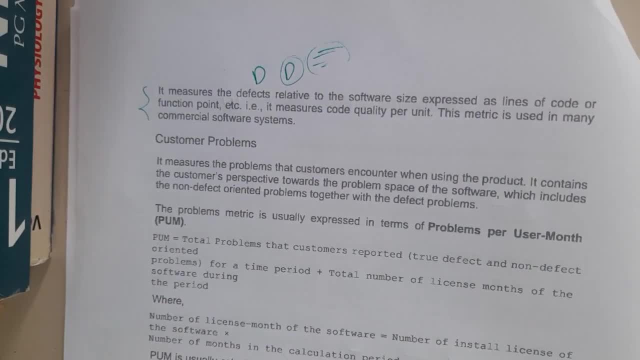 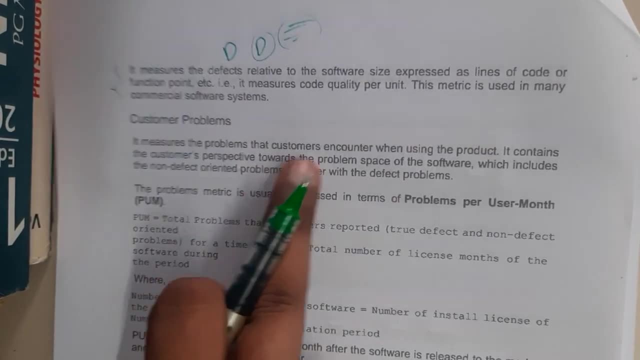 will be measuring here, guys. so in lines of code, how many defects are there for that much lines of problems. but we will be using it in a way which is uprising, but in a way which is growing. we will be measuring it, okay. similarly, customers, a problem? okay. so it measures the problem, that customer. 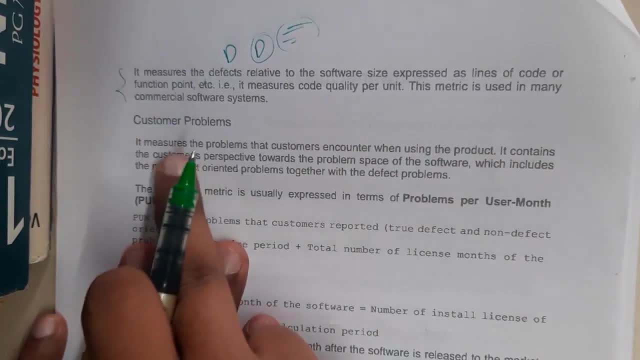 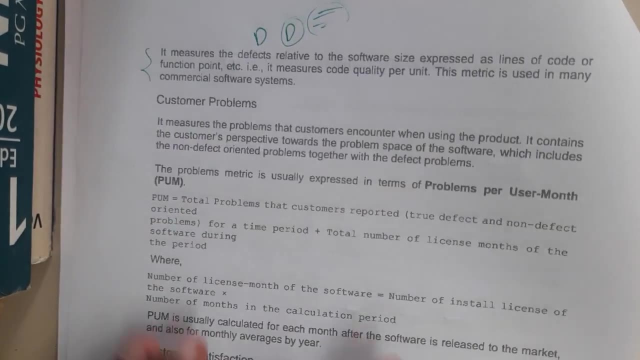 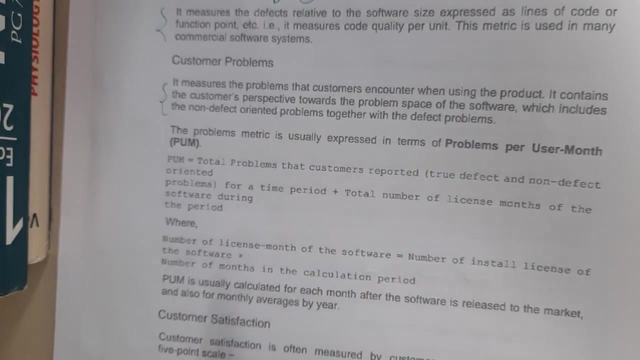 encountered when using the product. it contains the customer perspective towards the problem space of the software, which includes the non defective oriented problems through defection. okay, so basically these are nothing but the direct customer problem. so when you use an application, so assume that you bought a new pen and you noticed that the grip is not good. so those kind of defects. 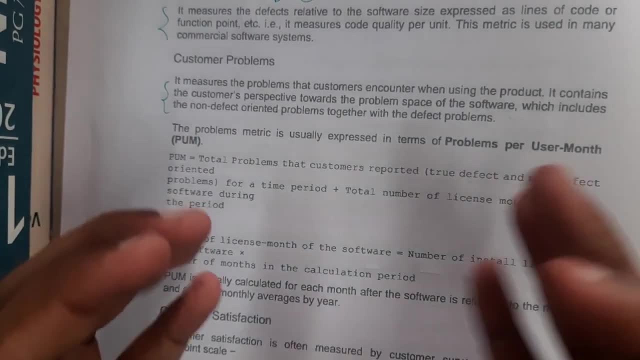 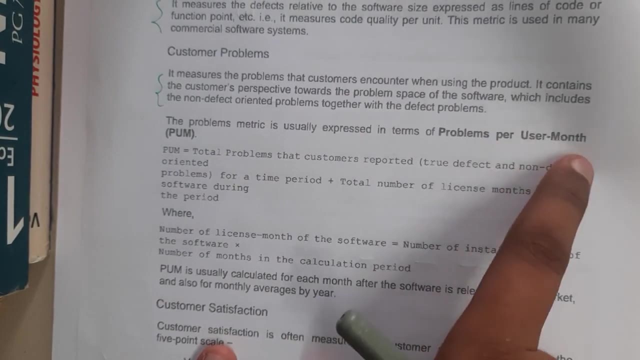 are prone, right? yes, so these will be intimated. so those all will be written in this matrix. okay, the problem matrix is usually expressed in terms of a problems per user month. okay, so that's nothing but pum. so these are some formulas, guys. i don't know where exactly we'll be using these formulas. 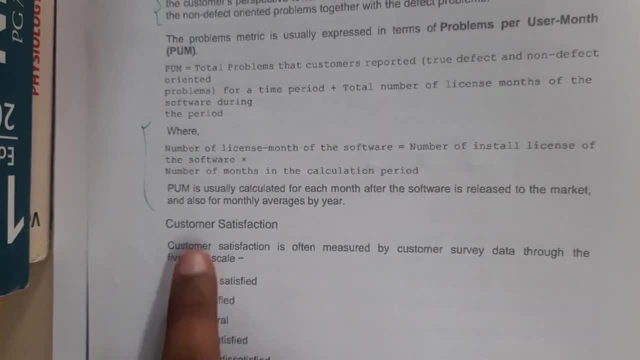 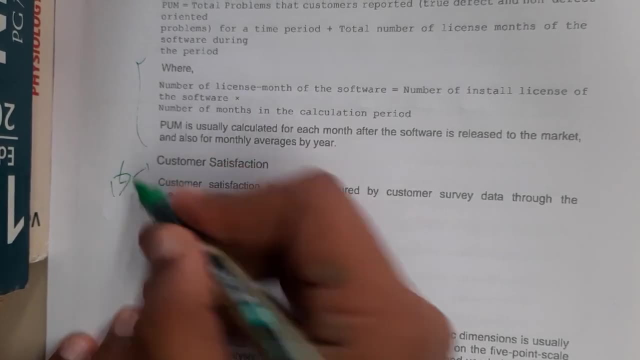 but please go through them once, okay, yes, okay. so the last fourth way is nothing but customer satisfaction. so this thing i hope everyone knows, right, so we'll be giving some reviews, right. so whenever a delivery, some delivery, food delivery or any kind of amazon delivery or anything is, 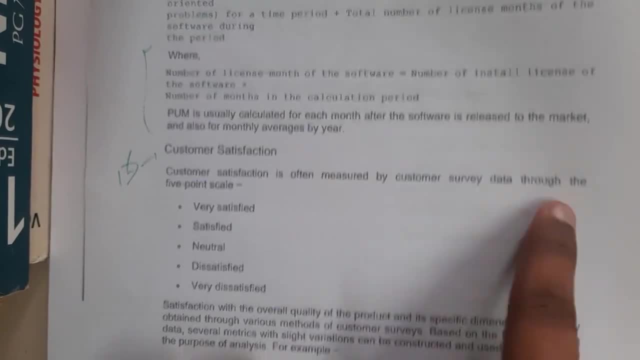 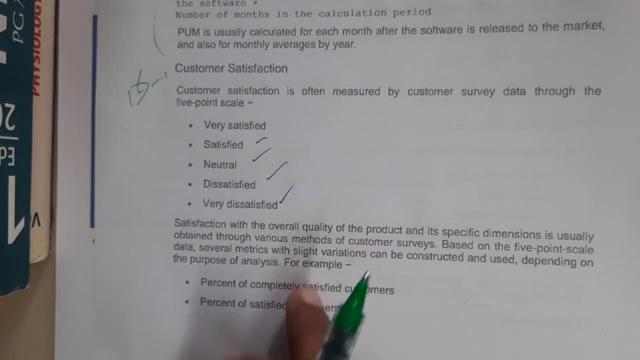 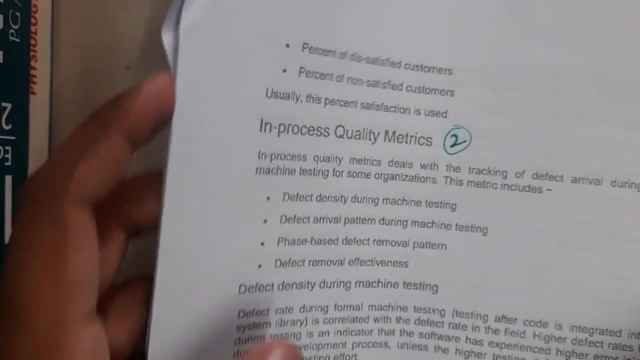 done. we'll be giving some reviews, so customer satisfaction is often measured by the customer survey through five points. that is nothing but very satisfied, satisfied, neutral, dissatisfied and very dissatisfied. okay, yes, so based on these percentages also, we'll be deciding some kind of factors. okay, yes, so i hope everyone got some basic idea about the first type. that is nothing but.